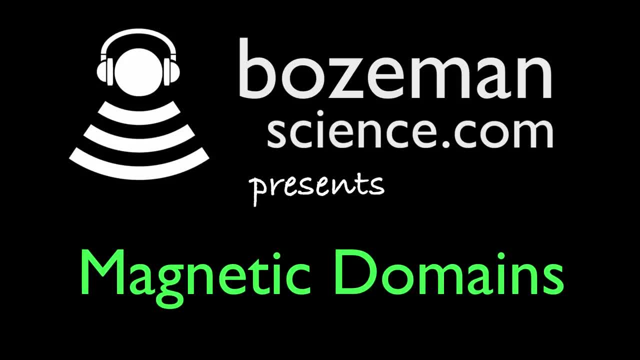 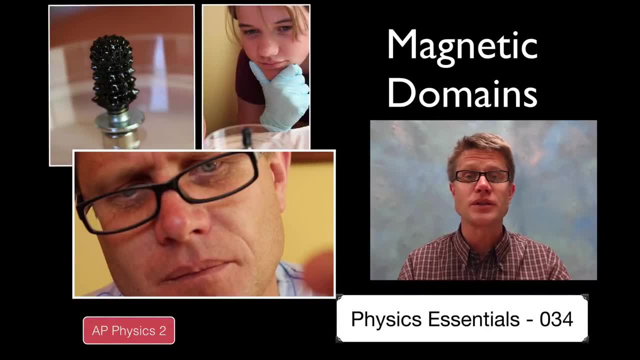 Hi, It's Mr Andersen, and this is AP Physics essentials, video 34. It is on the magnetic domains. In this picture right here, my daughter and I are both playing with ferrofluids, which are tiny little liquid magnets that can respond to a magnetic field, And so in this video, 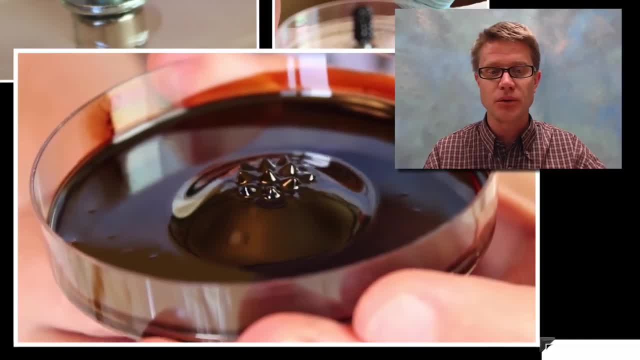 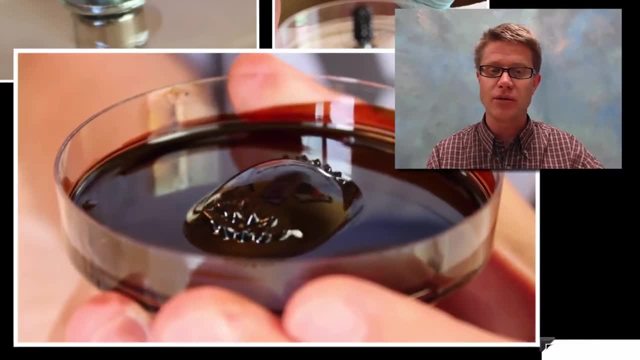 what I am doing is I am taking a magnet, holding it underneath the ferrofluid, and you can start to kind of visualize these magnetic fields. I can then turn it sideways and you can even see the north and the south pole, And so these tiny little ferrofluids are made up of these. 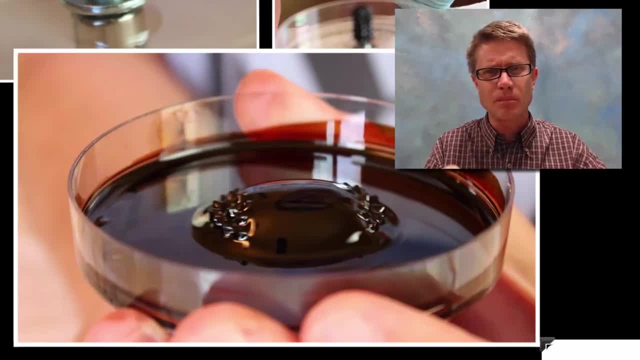 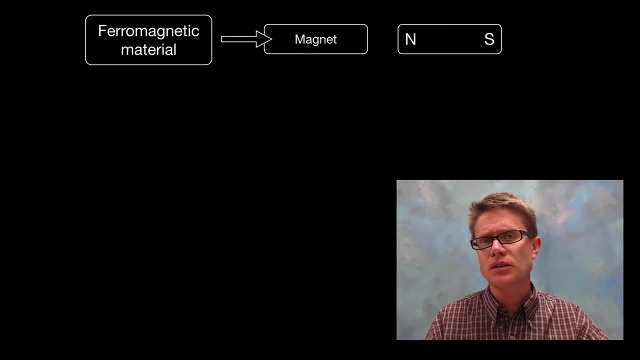 hundred angstrom, little magnetic domains, which are tiny magnets within the magnet itself. And so if you have ferromagnetic material in the form of a magnet, what you are going to get is a north pole and a south pole Again. you will never have just a north pole by itself. 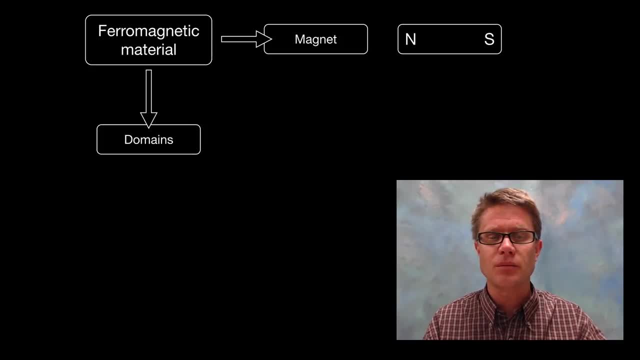 or a south pole by itself. But if we were to look inside that ferromagnetic material, we would find that there are these magnetic domains which you can think of as tiny little magnets, And each of those tiny magnets have their own tiny little fields. And so if you 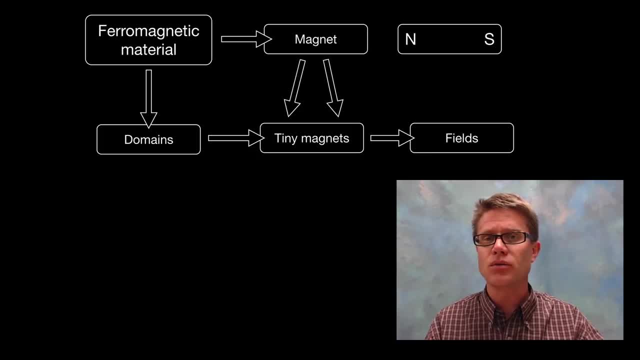 break a magnet in half. have you broken it? No, You have just created two magnets. And you could keep breaking it in half, over and over and over, until you get to the level of these tiny magnetic domains. And if these line up, if they align, then we have got an. 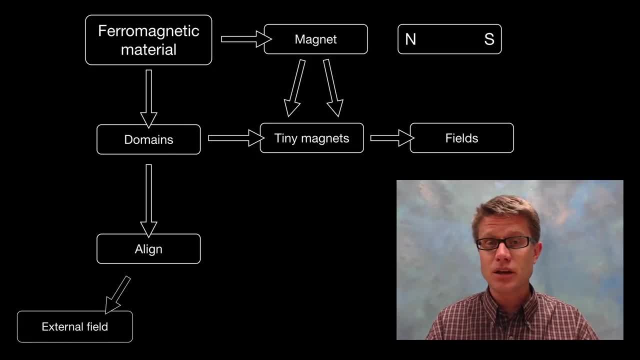 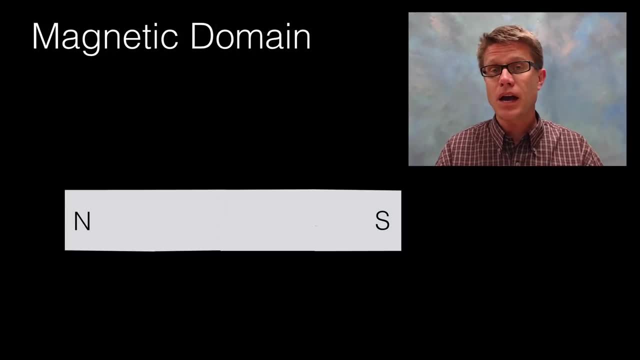 overall ferromagnetic material And they can do this by putting them inside an external field, Or sometimes it will just spontaneously Or naturally occur. And so if we have a bar magnet, it has got a clear north and a south. we can make sure that it is magnetized by holding a compass up on either side And you 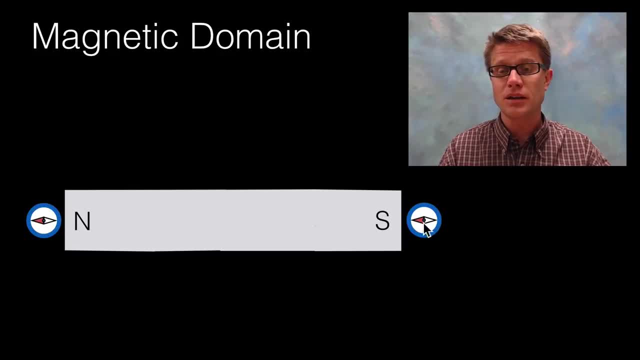 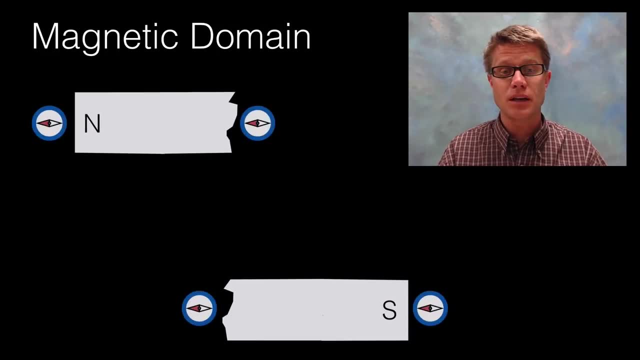 will find that the south end of the needle points to the north end of the magnet and vice versa. down here Now, if we break it in half, that bar magnet in half, what have we done? Well, let's use our compasses again. If we put them on either side, what you will? 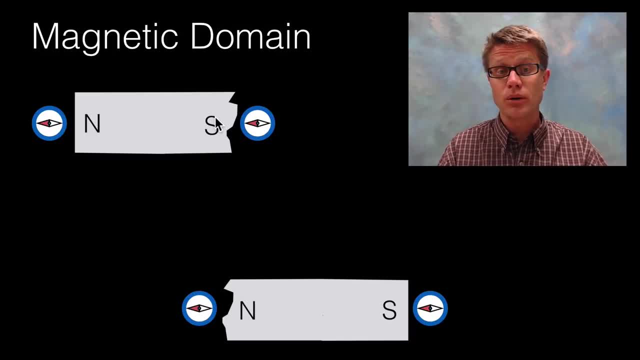 find is that we have now created a south pole at this side And then we have created a north pole up here. So it could do this again and again, and again, and we would just keep making smaller and smaller magnets. So there must be magnets within the magnets that are causing. 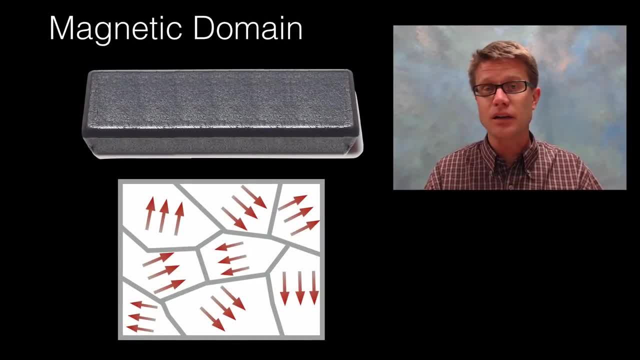 that magnetism, And so you can think of it like this: In a block of iron we have got all of these domains which are going to be tiny magnets inside it, But if the whole thing is not magnetized, they are going to be pointing in every rich direction And they are going. 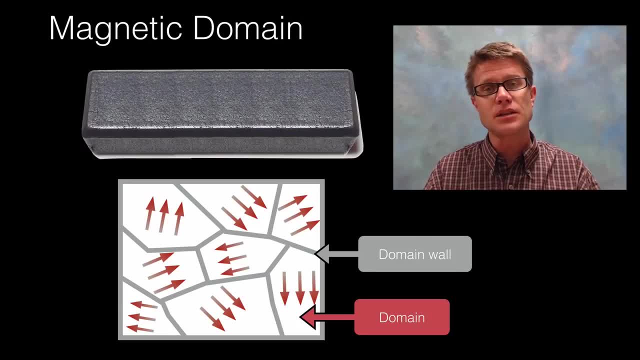 to be separated by these domain walls. And so if you take something that is not magnetized and you magnetize it, what you are going to get is the selbst. When you cannot magnetize it, you do not magnetize it. Hurry up Faster, slowly, Faster, And then waking稍. 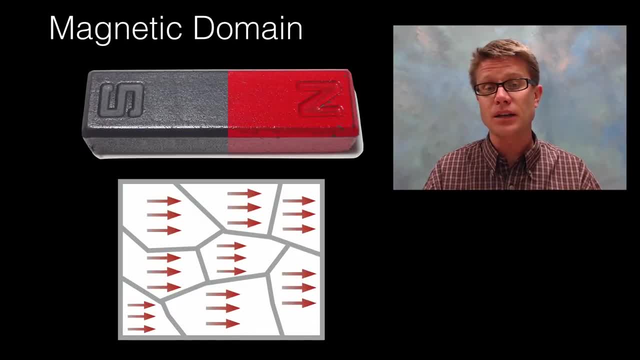 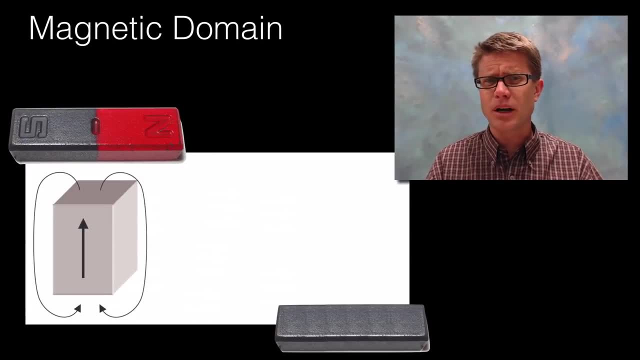 magnetize it. what you're really doing is you're lining up all those magnetic domains. If they're all pointed in the same direction, then you've magnetized that overall object, And so a question that might jump to mind is: why do we even have magnetic domains? What's? 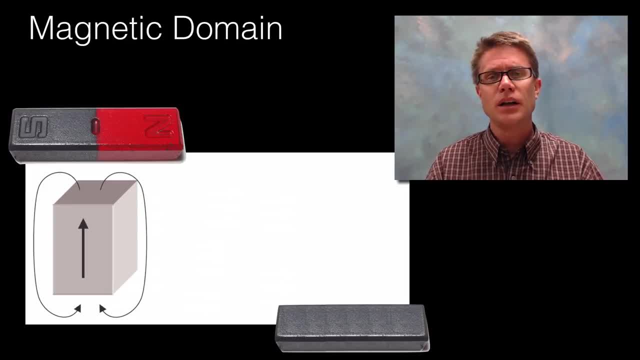 the purpose of having these tiny magnets within magnets? Well, it's an energy kind of question. So if we look at a magnet right here, it's creating these giant magnetic fields around the outside of it, And so what it's doing is using magnetostatic energy. is what scientists 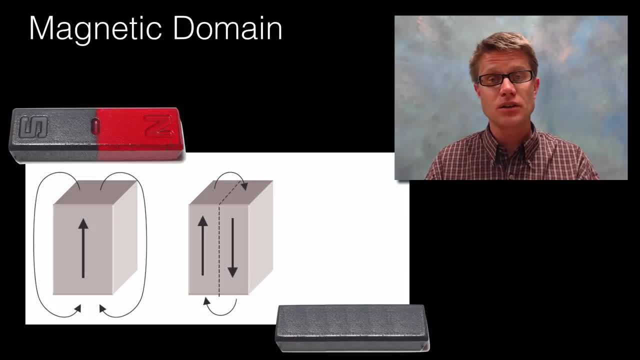 refer to it. And so if we can start breaking that down into smaller magnets, what we're doing is we're reducing the amount of that magnetic field and we're reducing the amount of energy, And so if we get a bunch of these domains, we've actually eliminated that overall. 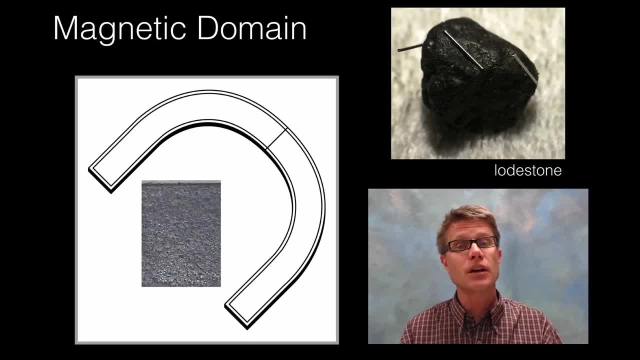 increase in energy, It's at a lower energy state. So let's say I want to go back again. Let's say I want to go from an object that doesn't have a charge to one that does. Well, this occurs in nature. Lodestone scientists and humans have known this for hundreds of. 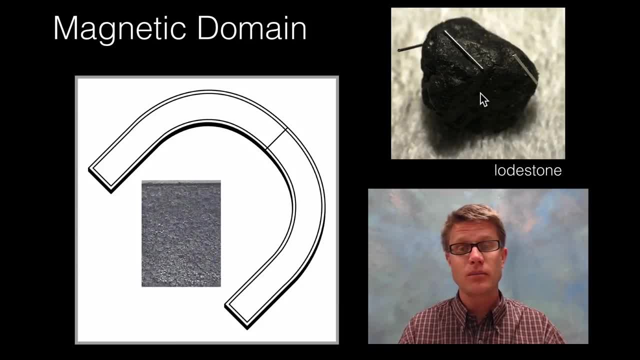 years are naturally magnetized pieces of magnetite. And so how does that work? Well, there's speculation that it could be that they're being formed, since we mostly find them on the surface of the earth near a lightning strike. But what it's doing is it's lining. 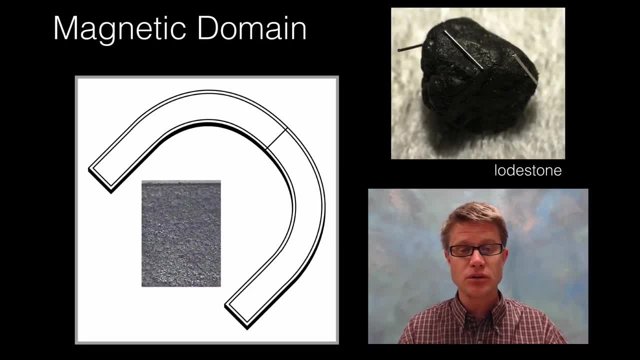 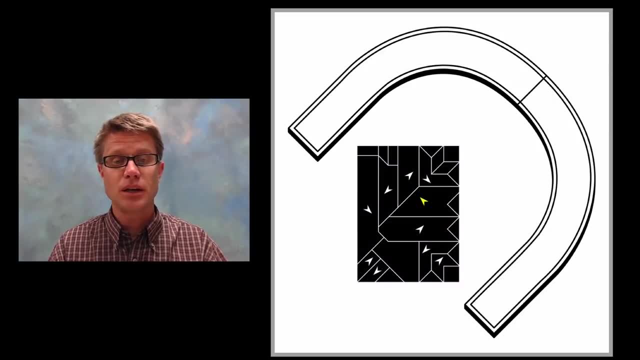 up these domains. If you want to do this in the laboratory, what you do is you take a chunk of some ferromagnetic material, like iron for example, and we put it inside an electric field. So we're going to put it inside a magnet And you can see at this point that we've got 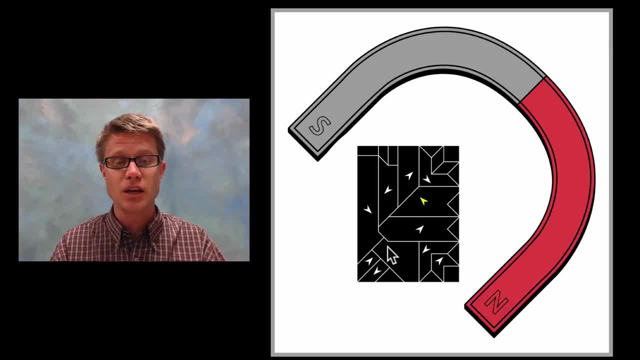 all these domains. again, they're much smaller than this, but we have all these domains and they're pointing in every which direction. But if we can apply a magnetic field to it, watch carefully right here. what happens if we let it sit there for a while is that we're.